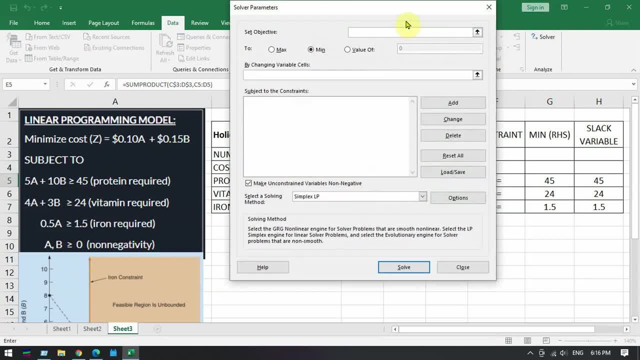 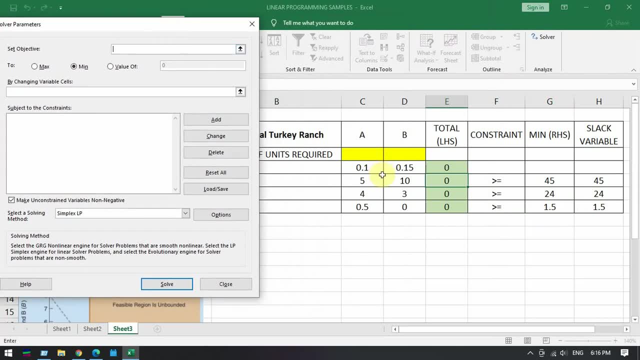 So let's start with the solver. We are going to find The value of A and B using this data. So our objective is: in this cell, okay for the total cost, It will be computed, And our objective is to minimize costs. 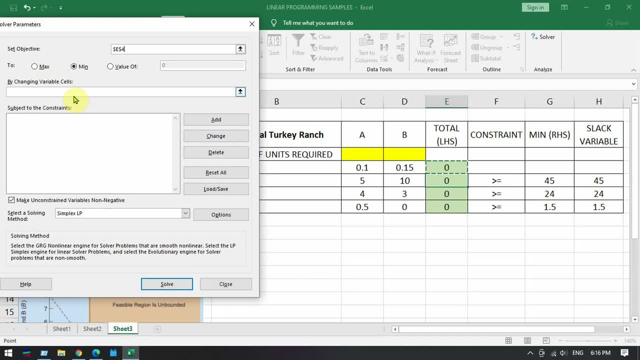 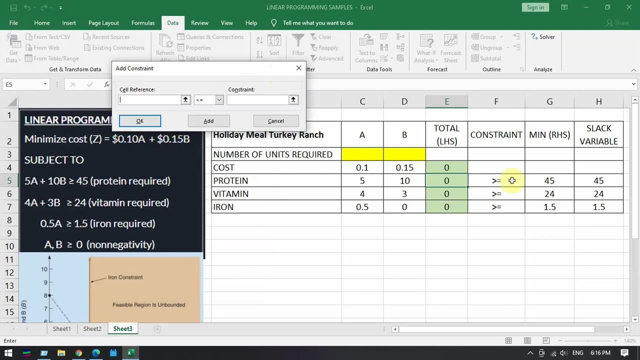 Okay. so I have already clicked here: minimize or min by changing variable cells. this cells- Okay. and then we have constraints. So we have three constraints here for protein, vitamin and iron And, as you can see here, all of them are all greater than or equal to, you know functions. 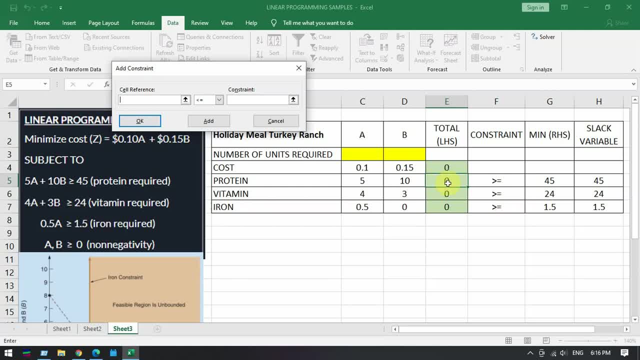 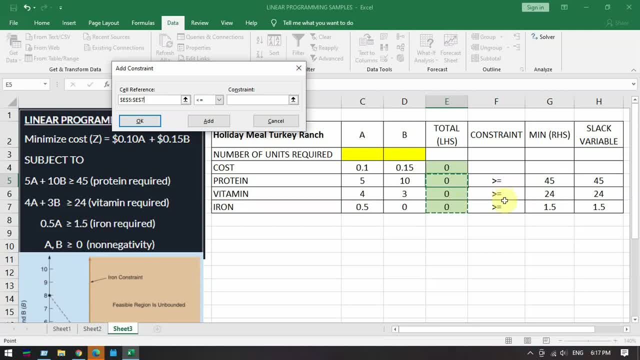 Okay, so this is for this cell. Okay, so this is for this cell. This is for the left-hand side. Okay, so this is for the left-hand side, And then the function is greater than or equal to, so this should be greater than or equal to. 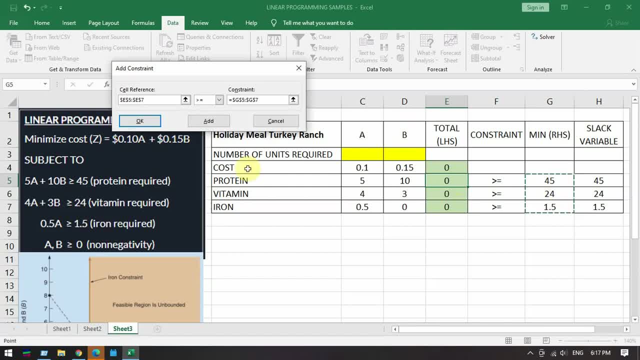 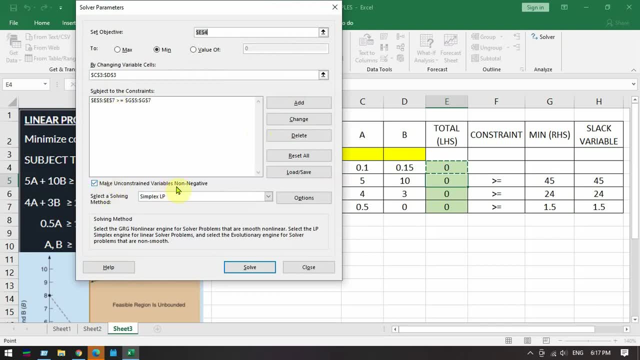 And our right-hand constraint is this: Okay, and then click Ok. And then click Ok, There we have it. And then we should click on this: make constraint variables non-negative, And we should solve it using the simplex linear programming. Okay, and then click Solve. 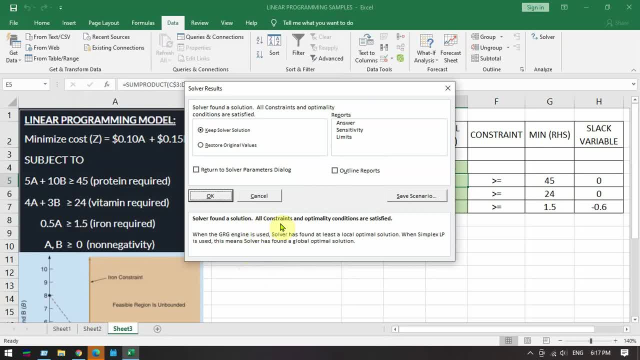 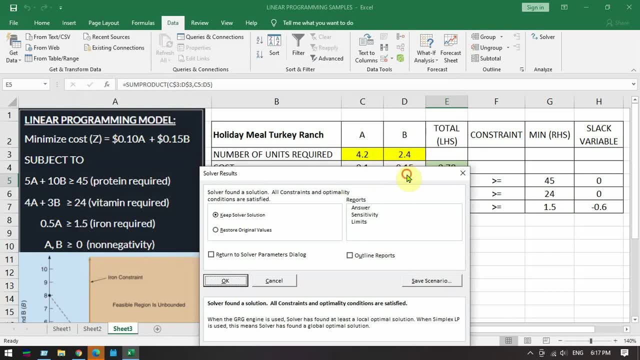 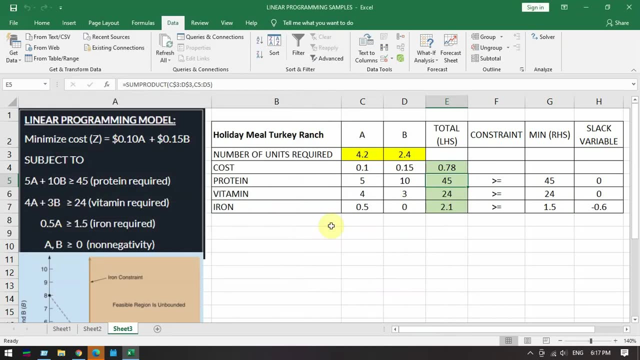 so it says here that solver found a solution. all constraints and optimality conditions are satisfied and the answer is 4.2 and 2.4 for a and b respectively. so we want to keep this solution, so we can just click. okay. so this is our first way or approach of solving our variables using the 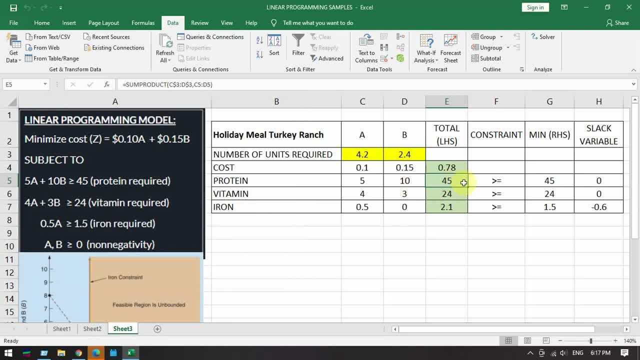 solver function okay, and this should be the constraints that we should follow, so that we will get the minimized cost of 78 cents per unit of okay for for both a and b together. so that's it, and then we can solve again using our mathematical functions. before we continue with the graph and to solve for our minimized 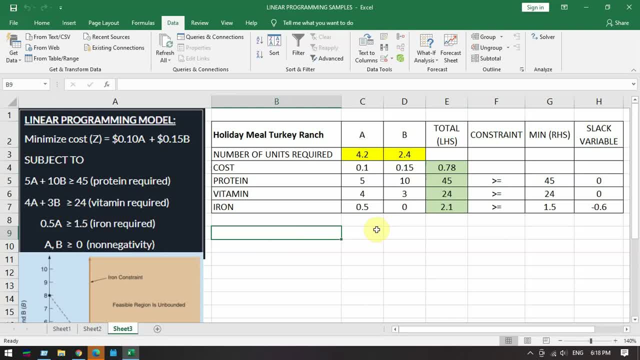 cost and also the right values for a and b. so we're going to use the formula of a mouth. so first let's go to our option, or the first point. okay, let's say point a, that we will have, uh, in our graph as one of our options. 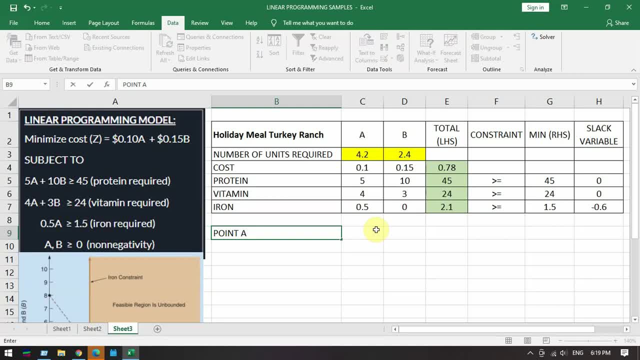 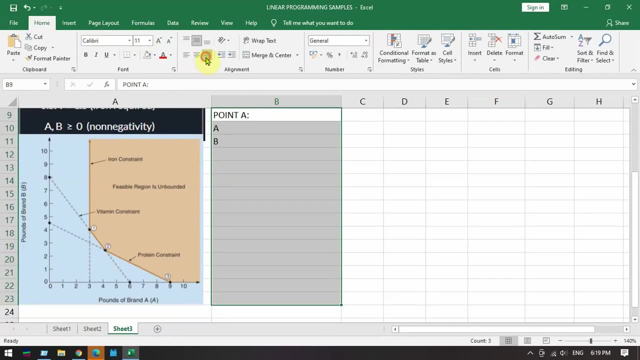 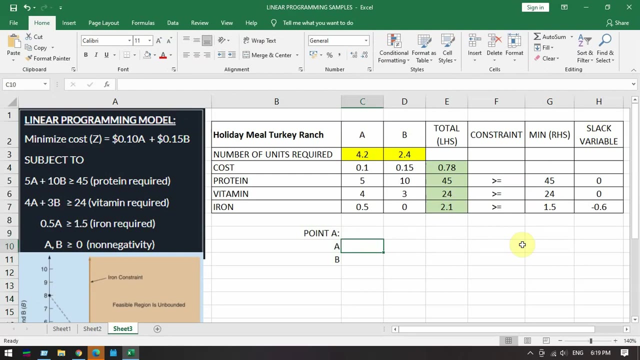 for the cost, for finding the minimized cost. so for point a. so of course we will have a and b, so let me just fix the format here and have them all here, okay? so for point a, we'll have um, protein and vitamin. that's right. this is for where protein and 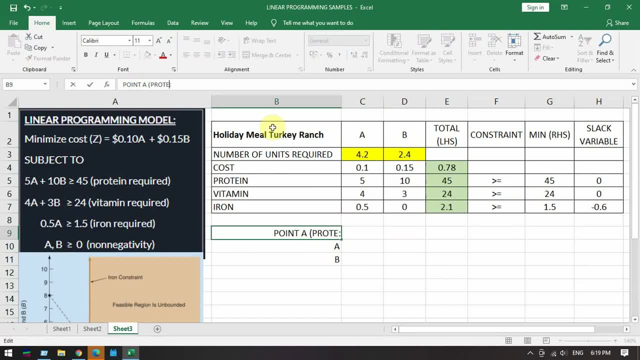 and vitamin will intersect. and to do that- we highlight again ourselves- so we need to fill up with a and b and we- and to do that we highlight again ourselves- so we need to fill up with a and b and we use our matrix, multiply function and then M inverse, so this is for protein. 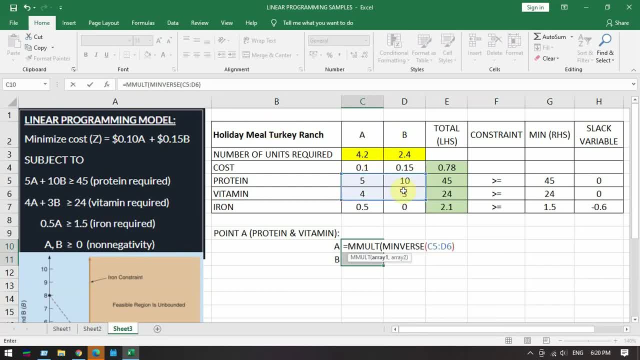 vitamin. so we do this comma and then our right hand side for protein and vitamin. okay. so again, we don't just hit enter, but shift control enter. so there we have it. okay, it's actually equal to this one. but this is: we're doing this in assumption that we still don't know our a and B values. okay, and our profit here. 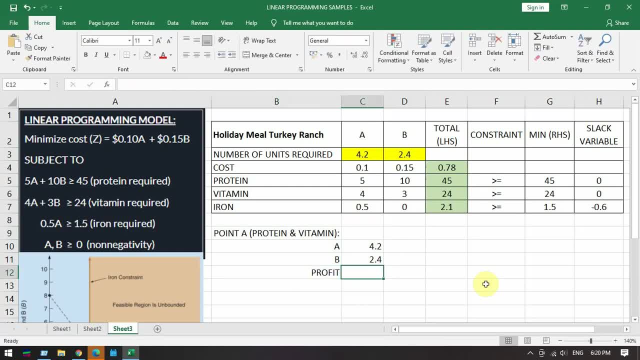 will be for point a will be this one times. I'm sorry that should not be profit, but let me just finish this formula. so this is cost, since we're talking about cost, right? and then the point B, though, we will have is for vitamin and iron. so let's have a and B. so again, 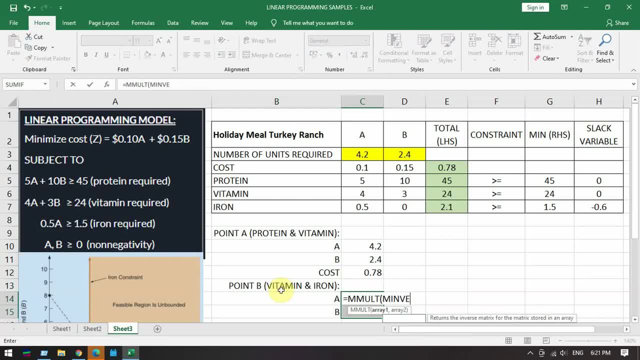 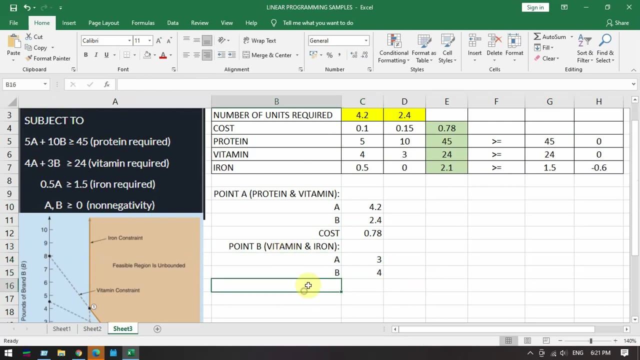 highlight, and then M, malt and inverse. then we have this close parentheses comma, and then the right-hand side, again shift control, enter, ok, and then the point B, point C, ok, which I'm sorry, let's first compute the cost, ok, so let's have it, let's. 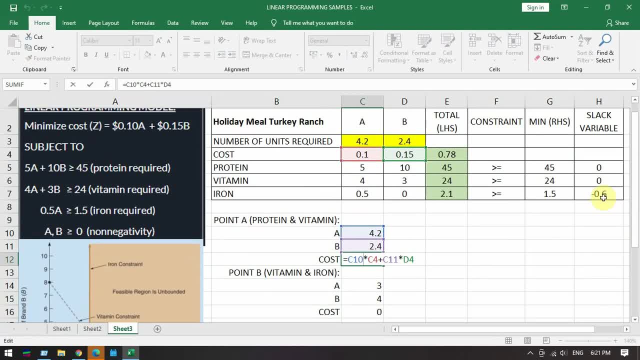 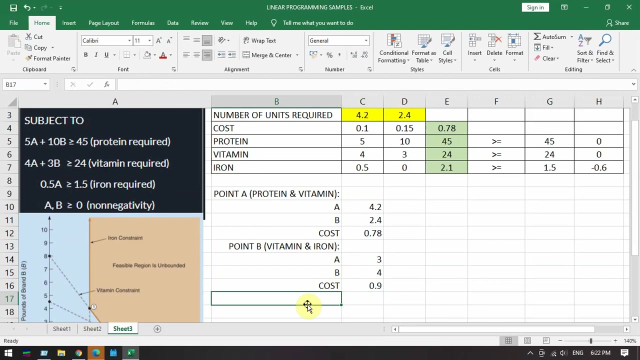 fix first the, the cells that should not move, and that is the cost per unit. and that is C4 and D4. so C4, let's put here dollar sign, so that when we copy we'll have you know the correct formula in here. so again point C, which will, or where protein and iron will meet in our graph. okay, so this lines: 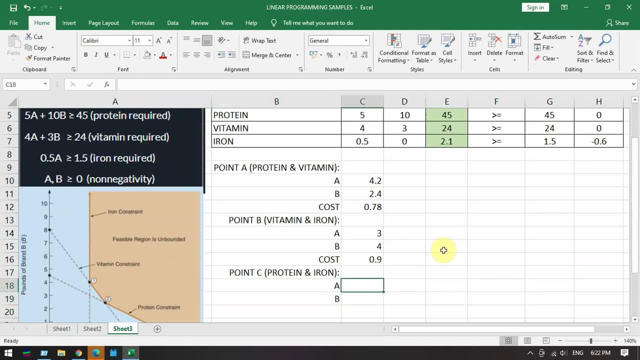 okay, so again highlight and malt and inverse and so oops, before that, sorry I forgot again. so we should make sure that this protein iron should be together first. okay, so that is necessary. so let's copy first the data. the same with the right hand side, okay? 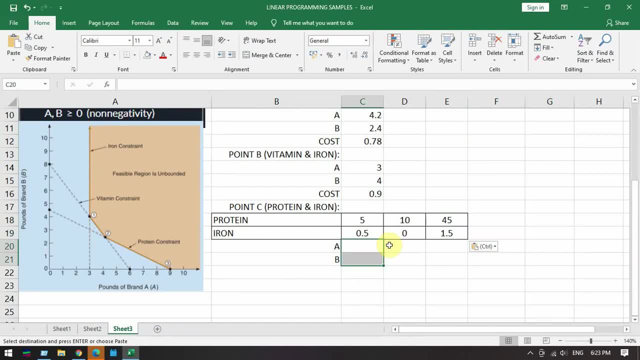 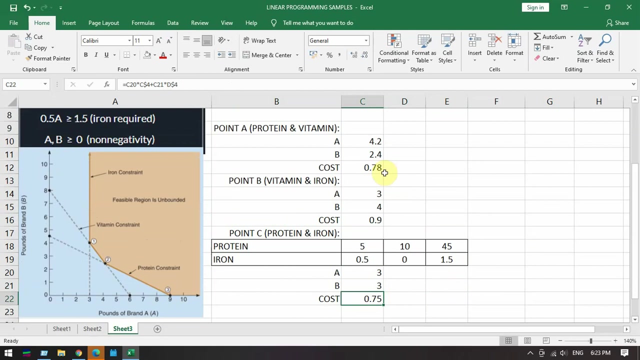 okay, okay, okay, okay, okay. so let's continue now. so this is M malt oops and malt M inverse. okay, so we're going to get this. and then we have this again: shift control, enter. okay, so this will be our third point, which will give us cost of 75 cents. so you actually notice, again we have 0.75 lower than 0.78, but our first 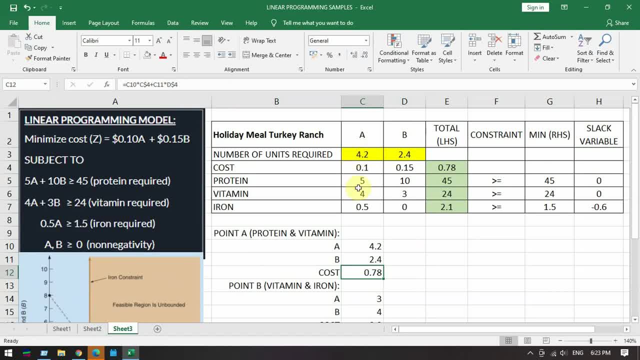 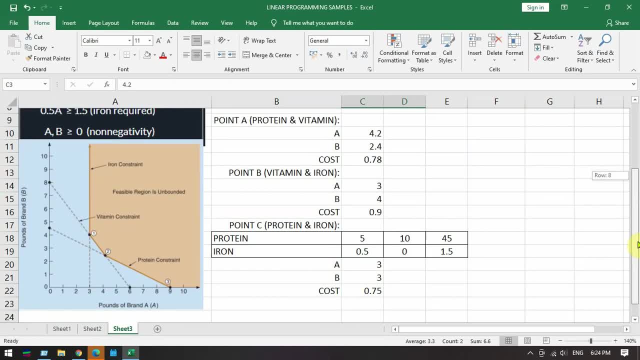 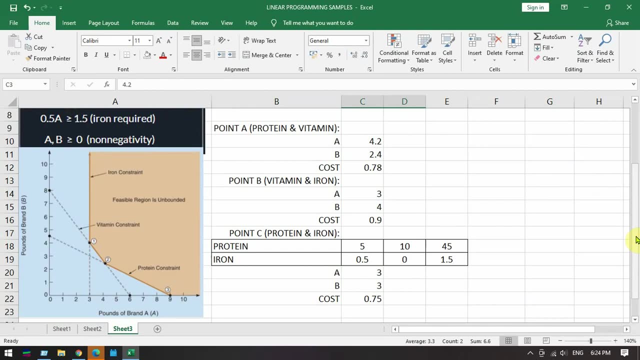 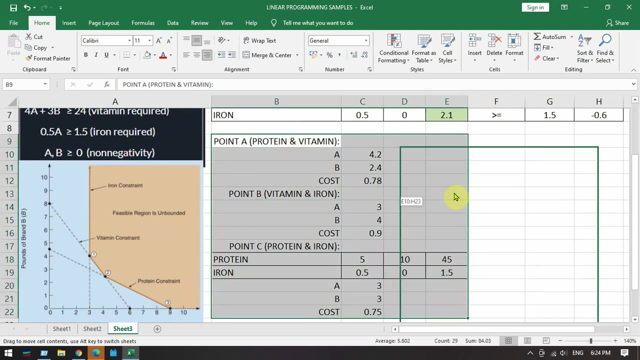 answer. using the solver shows that it is actually this values that it will give us the minimized cost. so let's see how it looks like in the graph so that we can actually identify or understand what happened. okay, so for the meantime, let's move this so that we can get our points for. 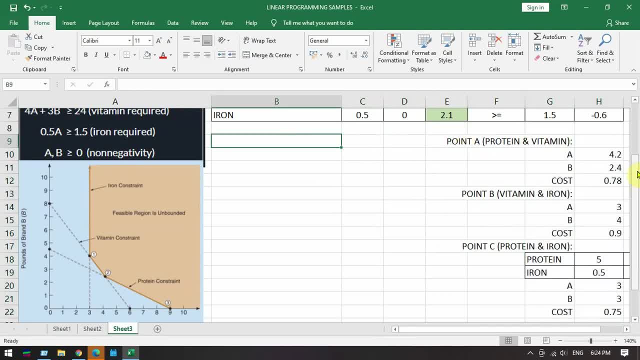 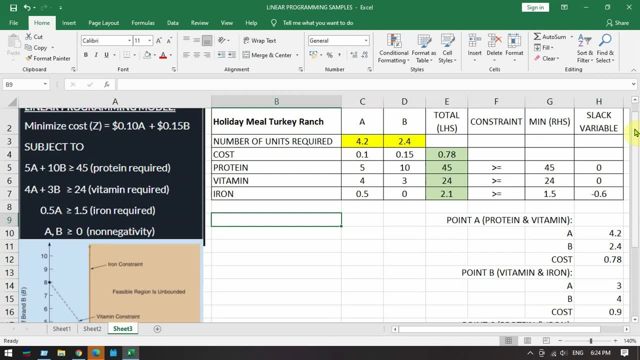 the graph. okay, so we're going to find out the points that we'll plot on the graph by using our constraints. okay, because it's our constraint lines that has to be plotted to the graph. so first we have for protein. okay, so that is using our stream points equation. so if a is, 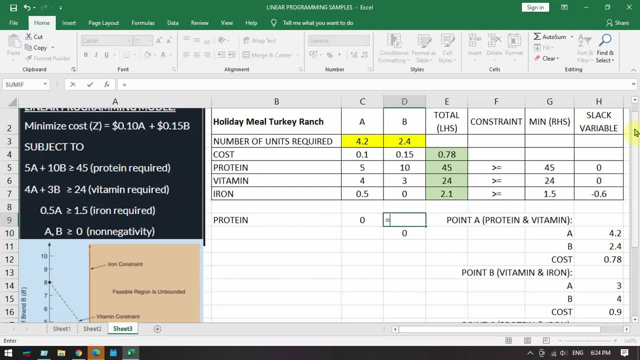 zero and if b is zero, so we're going to find out. so if a is zero, what is the value of b? that is 45 divided by 10, that is 4.5. okay. and for point a, if the that is 45 divided by 10, that is 4.5. okay. and for. 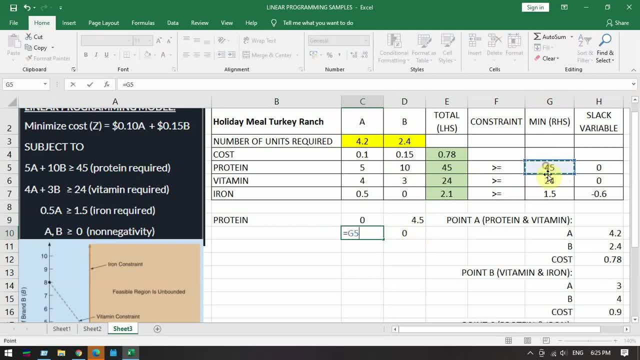 point a, if the value of b, that is 45 divided by 10, that is 4.5. okay, and for if B is 0, then that will be 45 divided by 5, right? so if we do this again to check if our answer is correct, so of course this is for protein, so we should. 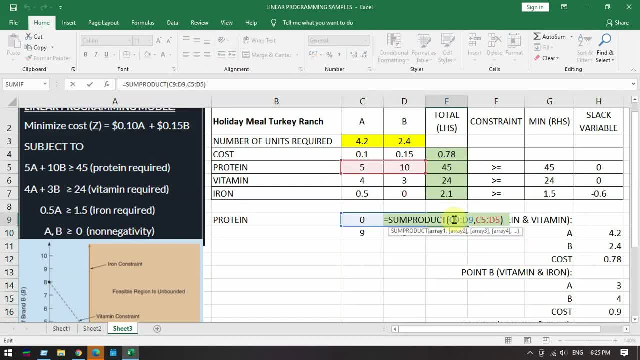 get there 45. so again, we don't want C5, C5 to move there it is, it's equal to 45. so our next point will be, or our next constraint line will be for vitamin. so that is, if A is 0, then our B will be 24. 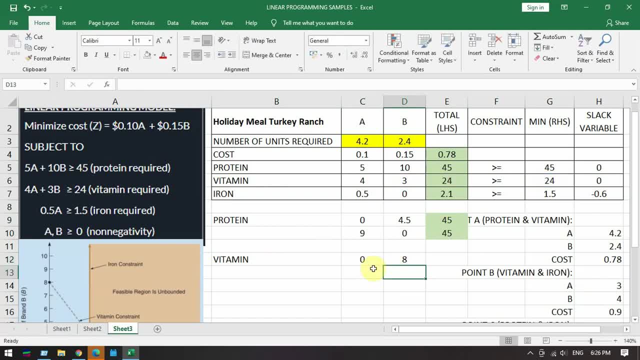 divided by 3.. That is 8.. So if B is 0,, then A will be 24 divided by 4.. Okay, So let's copy the formula here and let's just adjust. Okay, So that it will go to vitamin. There it is, So it should. 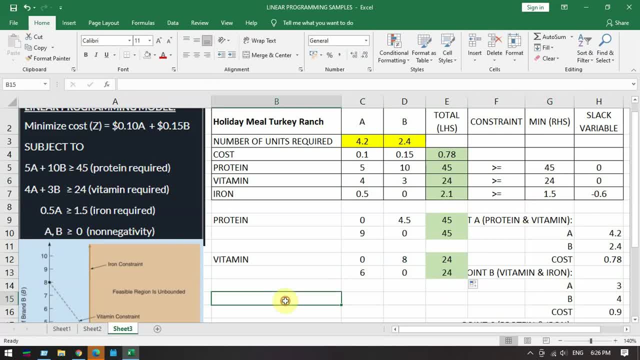 equal to 24 here, And then for our iron constraint line. So if A is 0, then B will be 1.5 divided by 0. So that is 0 also. So let's just change it to 0. And then, if this one is 0,, B is 0,, then 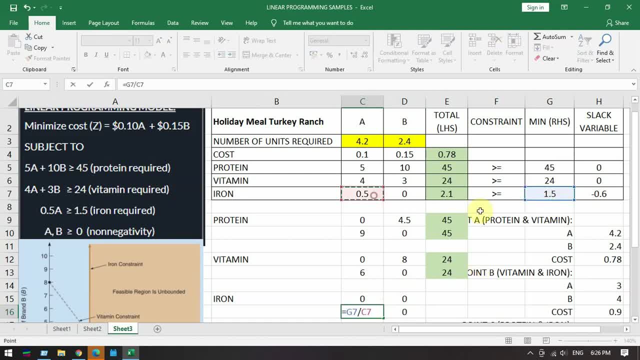 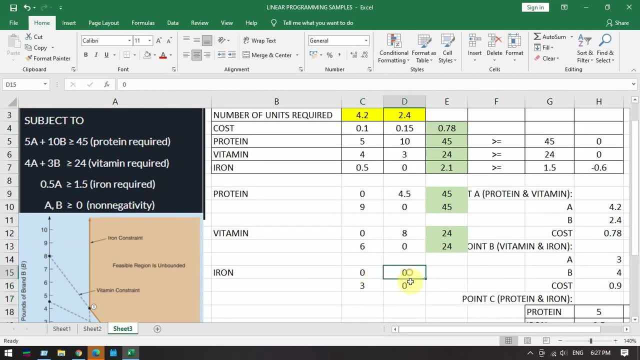 A will be 1.5.. 0.5 divided by 0.5.. Okay, So we only have one point in here, So later on we're going to adjust. Okay, So, make an adjustment for this one And, by the way, let's have this solve Right. 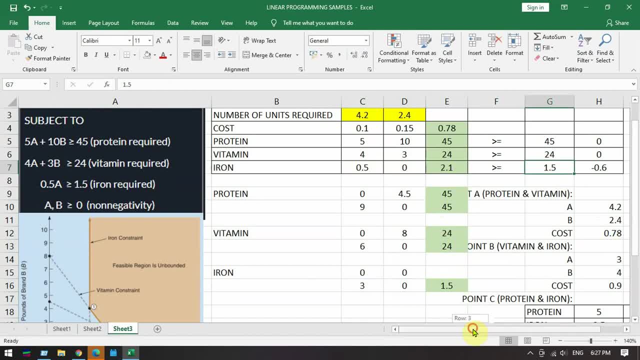 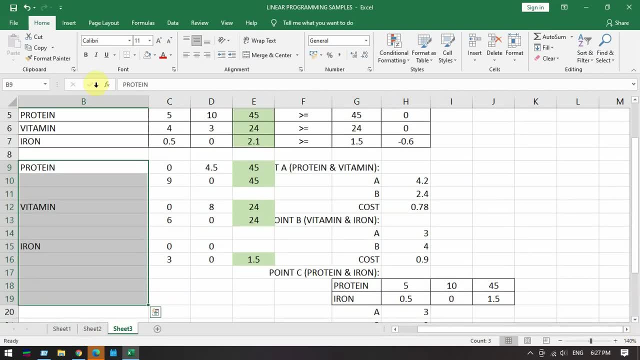 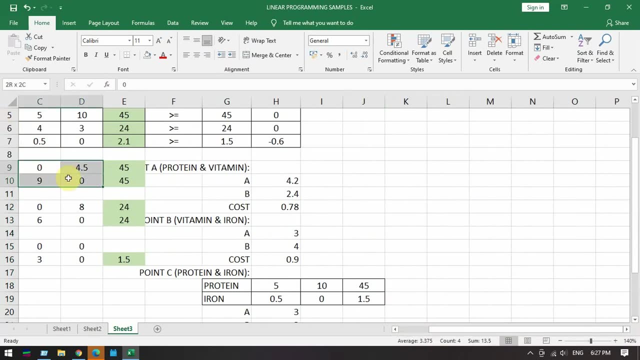 That's it. So it's equal to 1.5.. So we are now ready to plot our graph. Okay, So let's do this on the right side, Sorry, Okay. So for protein, let's start with protein. Insert Scatter graph with lines. 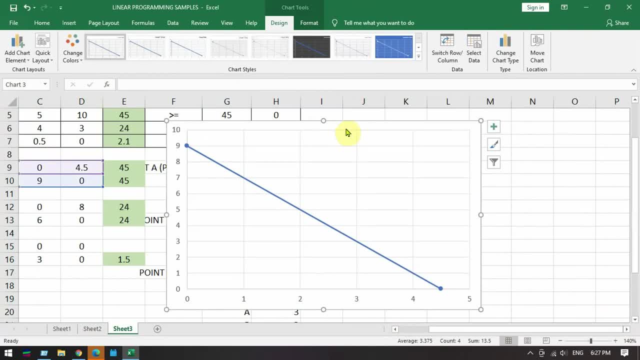 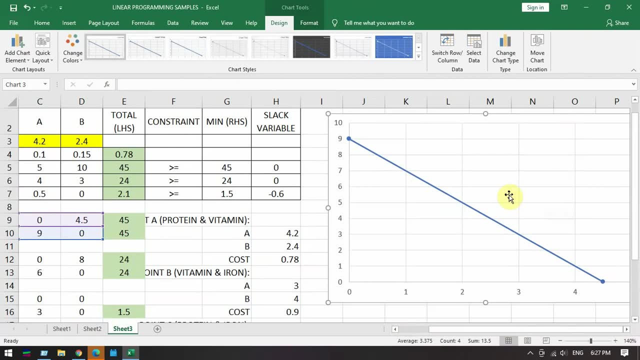 Straight lines. So let's just remove this chart line here. So, and then let's see if our points are correct. So our x-axis should have 0 and 9.. So we have to switch the row and column here, because the X data goes to Y and the Y data goes to. 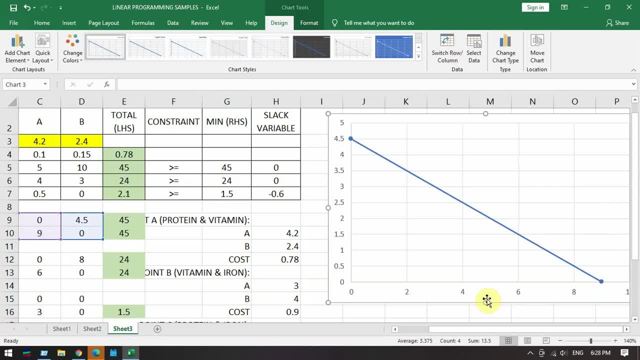 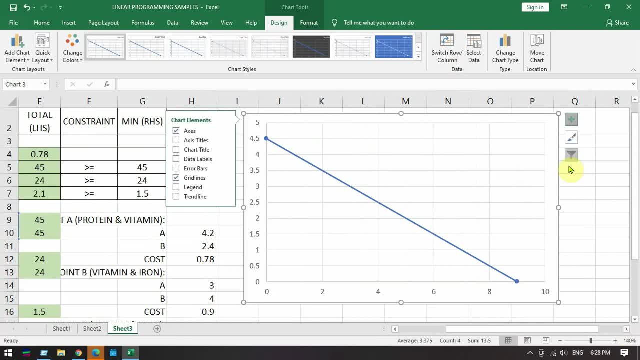 X, So let's switch here. So there we have it. And then let's just add a label so we know our lines, constraint lines, And I also would like to put the بال just to define it. And I also would like to put the بال just to define it. And I also would like to put the بال just to define it, and then they have a right here and a left there to create a boiled line in the first case. so what we need to do is to solve this, is to say you have to do triple milk and double milk with the N equals first. 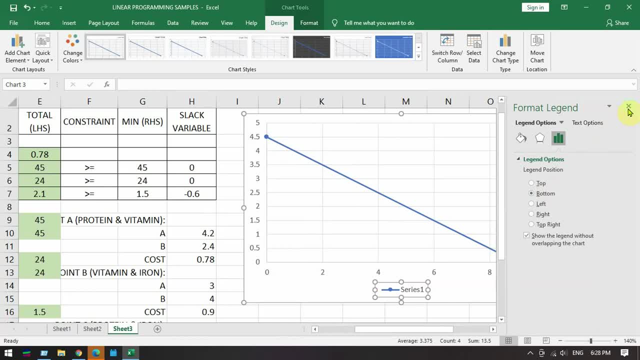 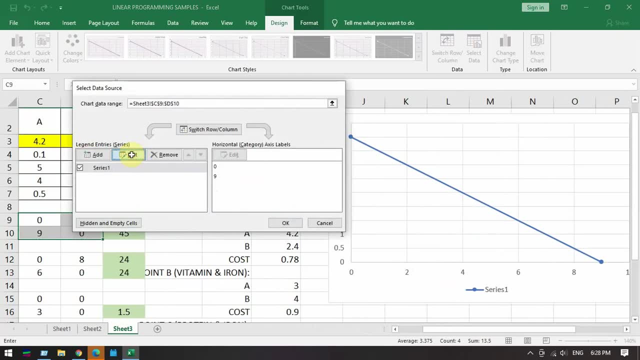 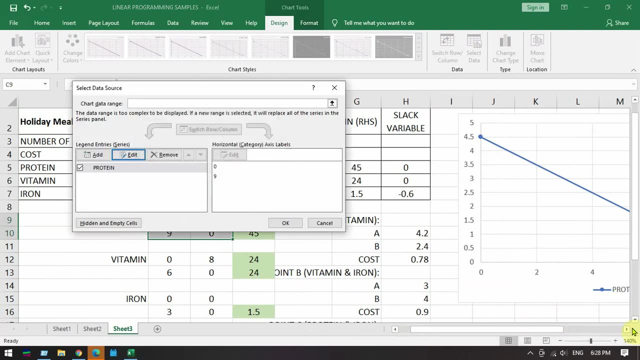 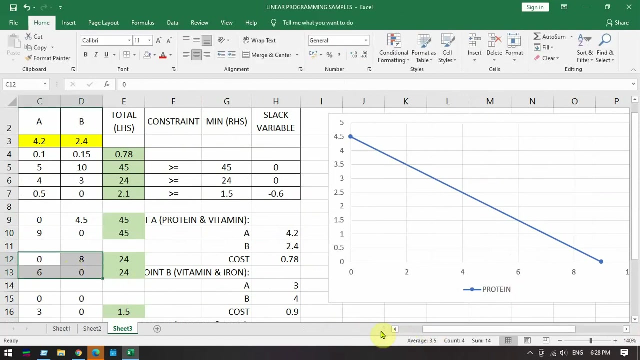 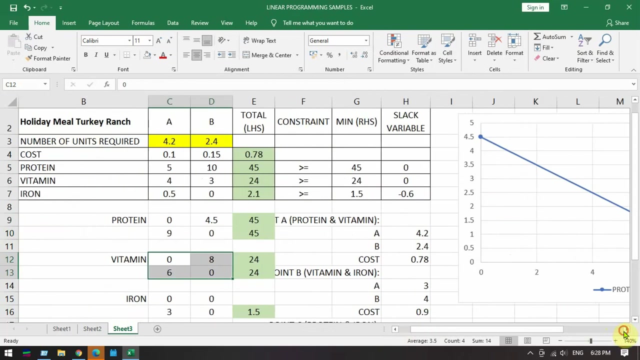 put this at the bottom. there we have it. so let's change the series data by editing the name from series 1 to protein. okay, that's it. sorry. so we see it's changed. and then we're going to add the, the one for the one, for what is this vitamin? so that is again select data and then add, so our 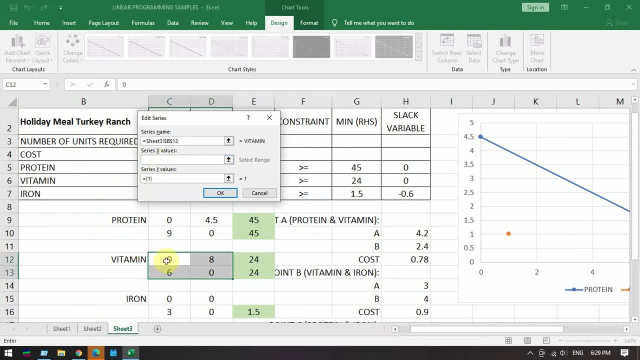 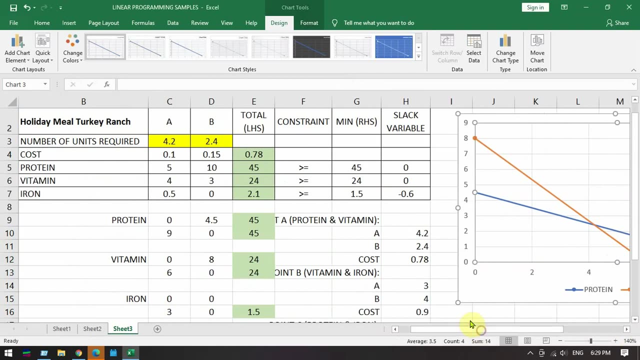 serious name will be vitamin. our X values will be 0 and 6 and our Y values will be 8 and 0. okay, so there it is, it's done, and then we will go. we are going to add iron again. select data: add iron- a serious name. X is 0 and 3, but we're going to change that later on, okay. 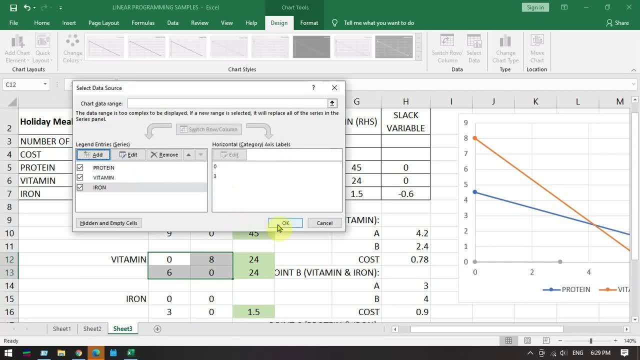 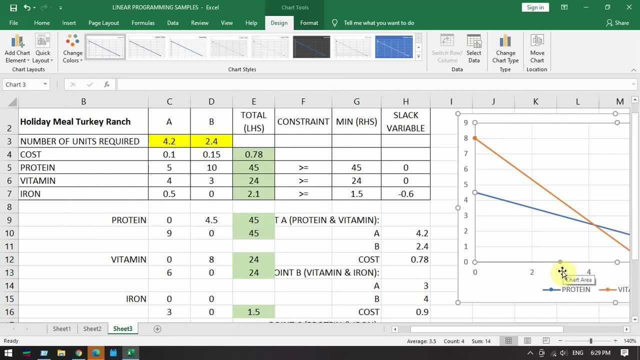 and this one right, and there we have it. so, as I said, we need to change the one for iron, the points for iron, so that we will get the desired line. okay, so our desired line is about. so it says that we should have greater than or equal to. so, since we're our 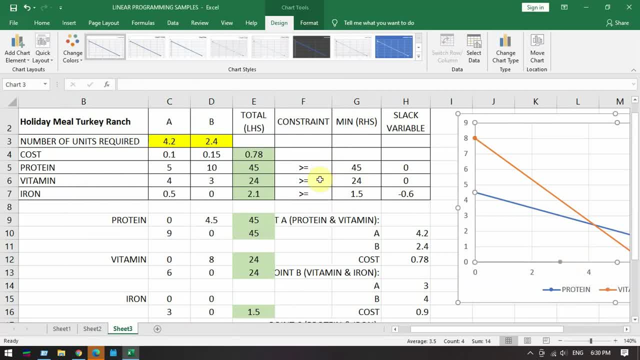 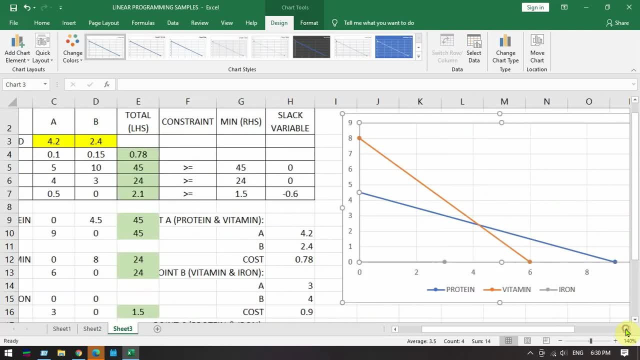 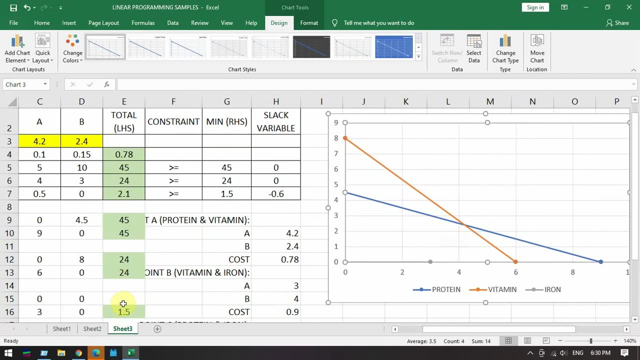 constraint lines are the minimums. so all of our the feasible area that we will get is everything on the right of our constraint lines, and the same with this for iron. so what we, what we're determining, and the minimum, so our line should tell us about the minimum requirement. so this time, what we need is: 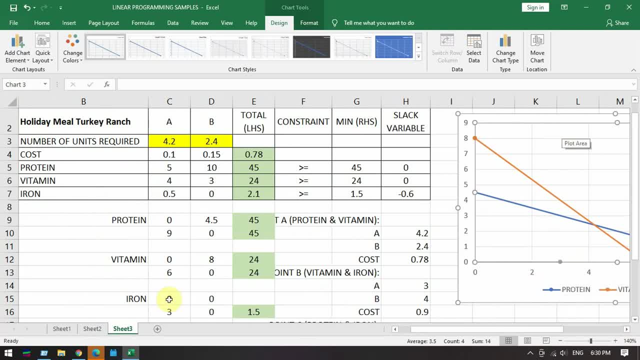 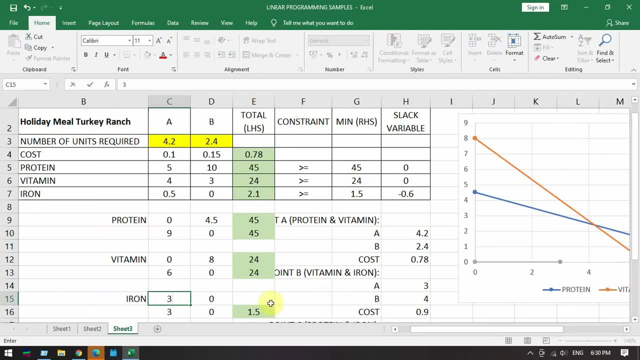 to make sure that this line will go straight up there. so we just make little modification here. let's put three, so our point just goes to point three in here. and for the y-axis let's use up to eight, so let's edit it to eight, so it's the y-axis that we will change. 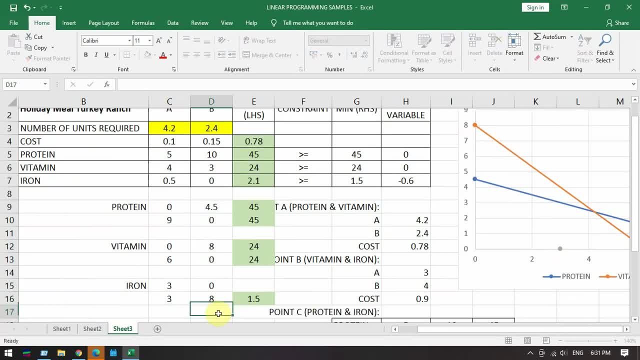 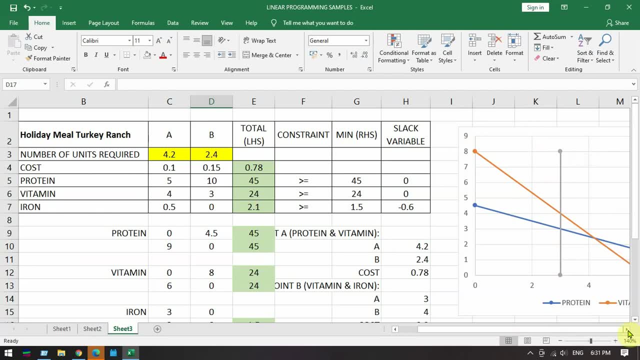 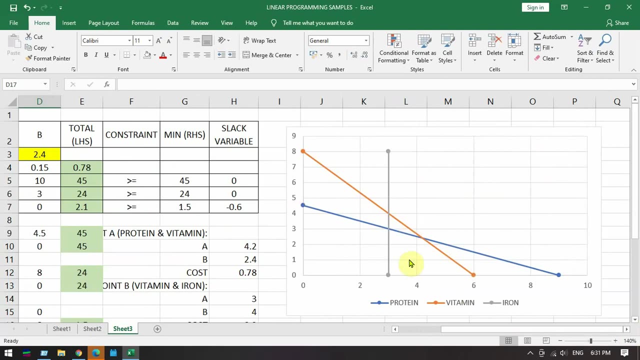 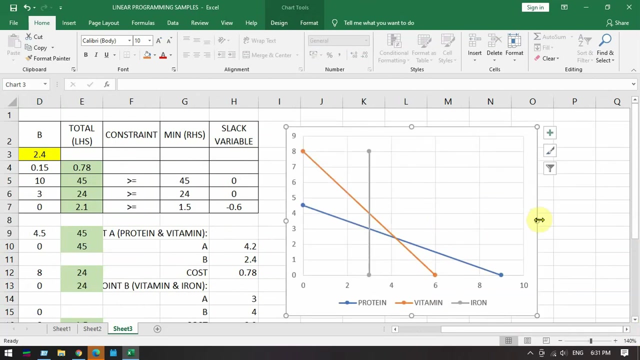 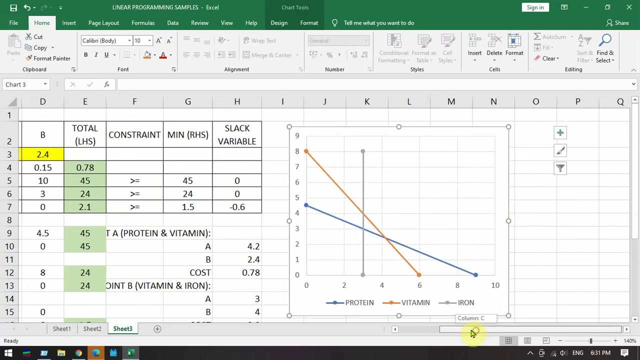 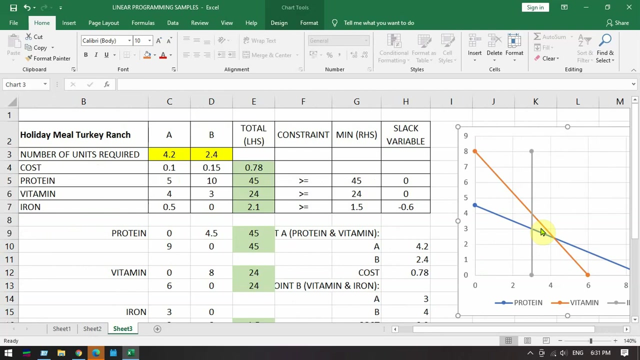 and that is eight. okay, so there, we already have the straight line. so we're done with this. okay, we already have our graph, so let's just fix the ratio of our graph so it will look nice and easy to understand. okay, there, we have it. okay, so let's understand now our feasible region. 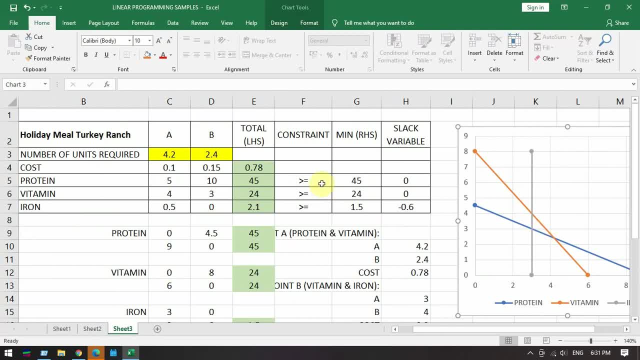 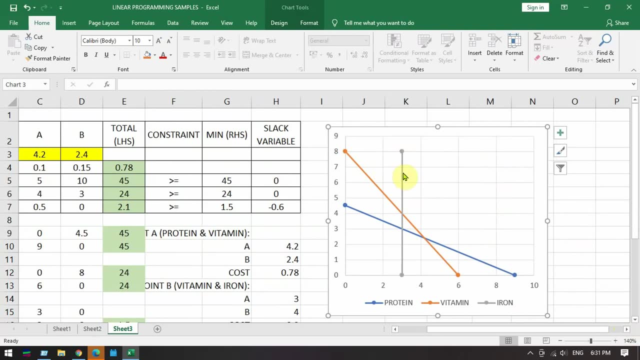 okay. so in our formula for constraint we say that all this, all these lines, are our minimum, okay. so, meaning, our feasible region should go beyond this lines and that will be this: okay, all the way up or all the way outside, okay, so this will be our feasible region. so with that, we are now ready. 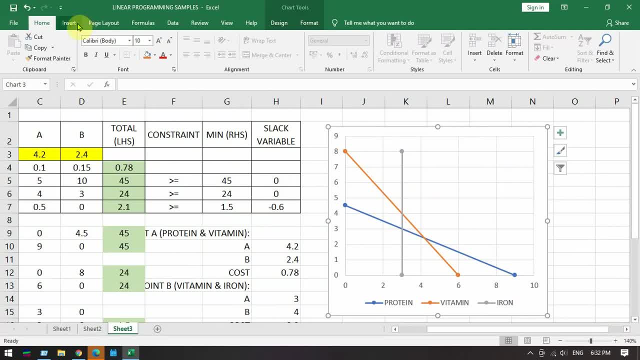 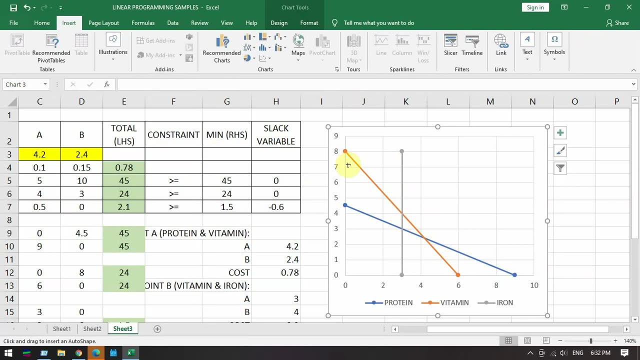 to determine our minimized cost or optimal solution. so before that, let's first put a shade by adding a shape here. okay, all right, so let's just since we cannot, so this will be unlimited. okay, so let's just since we cannot, so this will be unlimited. okay, so let's just since we cannot, so this will be unlimited in this case, right. 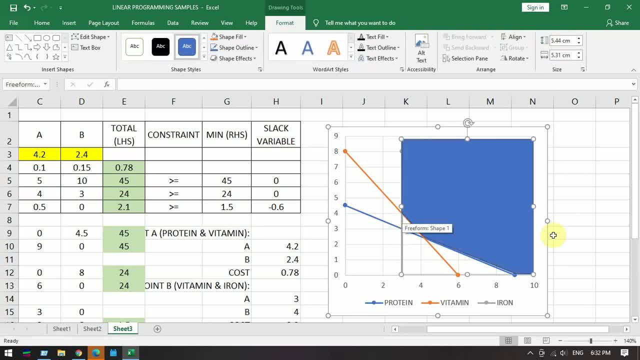 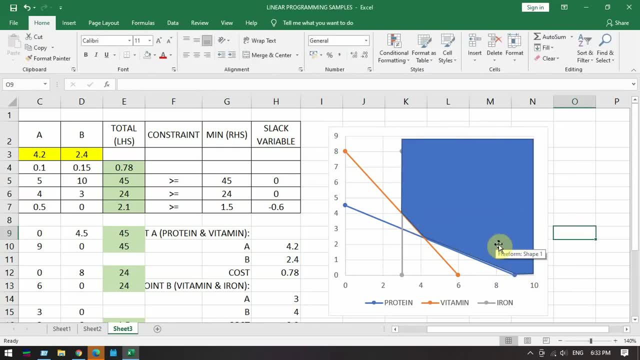 okay, there it is. so the shaded part is our feasible region. I haven't really have it exactly here, but this shaded part is our feasible region, so our optimal solution will lie somewhere in here. okay, and we're talking about cost, so, and our goal is to minimize the cost, find the 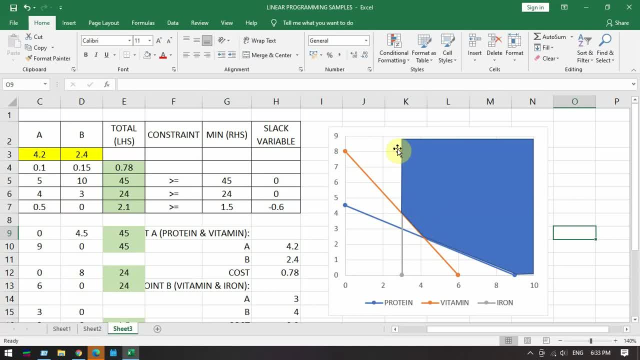 minimized cost. therefore, our optimal solution will actually lie along the border or the corner points, one of the corner points of our feasible region, okay, and somewhere here, you know, near the zero or outside our feasible region. so in here we're going to use what we have actually solved for the value of a 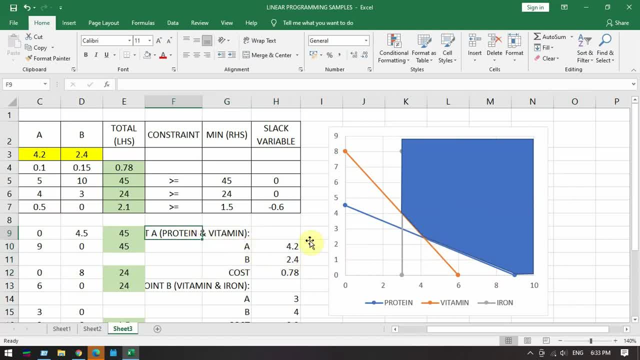 and b for the different points. so our point a, let's determine where our point a es, because this points that we have calculated earlier are the various options for our optimal solution. so point A is where protein and vitamin intercepts, and that is four point-ooky, and vitamin intercepts, and that is four point-fi. 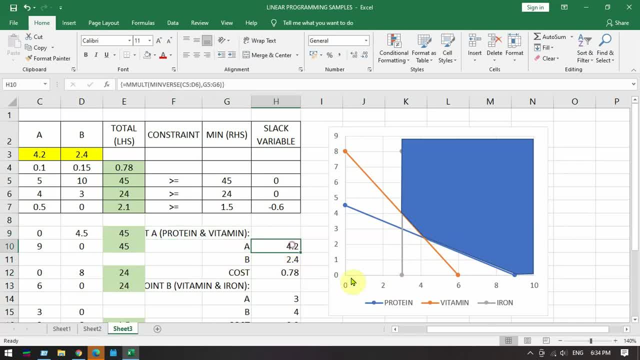 so point-a is where we calculatease the value. this thus an optimal solution, which which will result a priority. this is this one from 1 and B, or titel, and that is this one from 1 and B, or titel. 4.2 of A. so this and 2.4 of B. 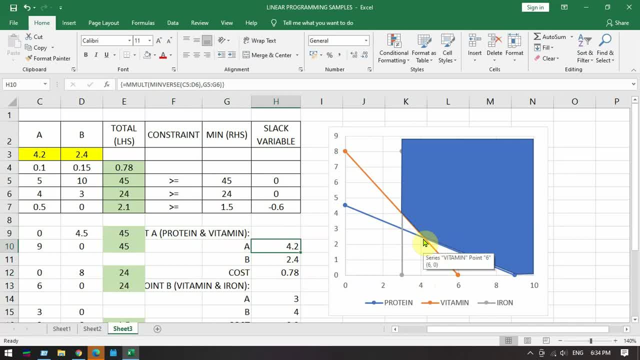 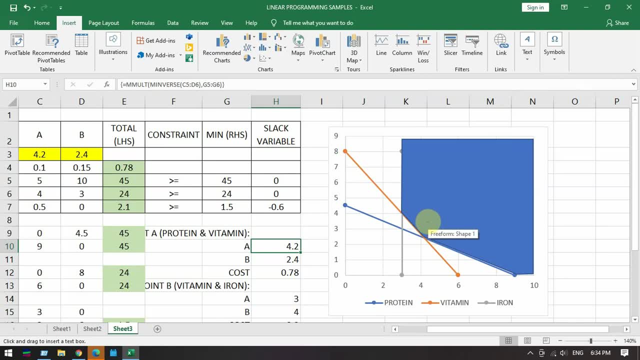 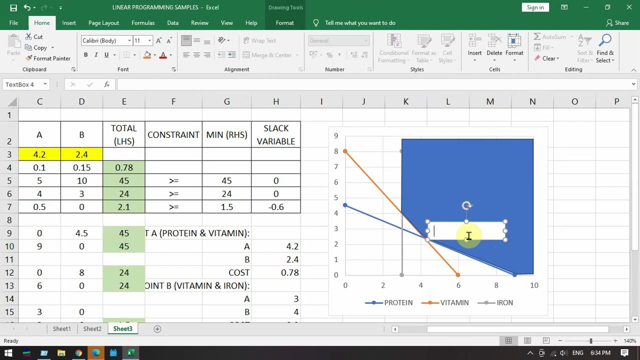 Okay, so this one is the one 4.A, So let's just identify that. Okay, so let me just do it here. So our minimize, our point A is, let's just put here the total minimize cost, And that is 0.78.. 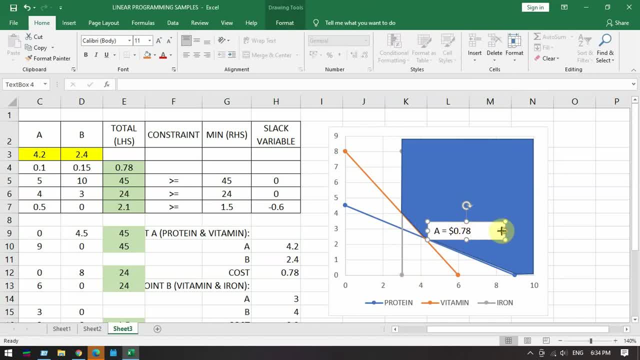 Okay, where our A is equals to 4.2, and B is equals to 2.4.. So our next point will be where the vitamin and iron constraints intercepts. So that is where A is 3, so here And B is 4, so here. 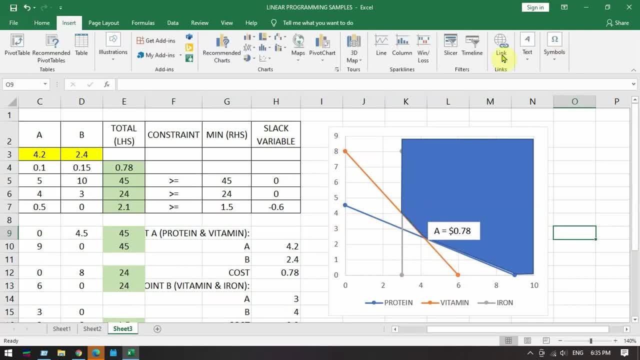 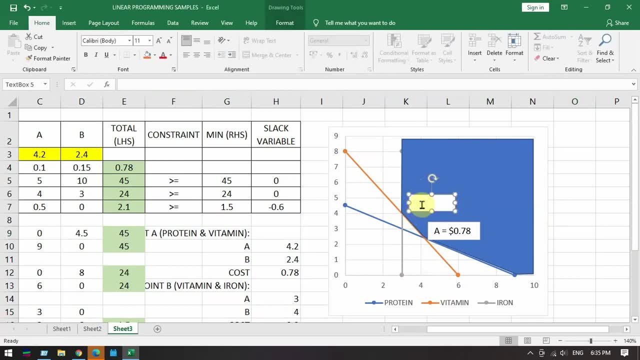 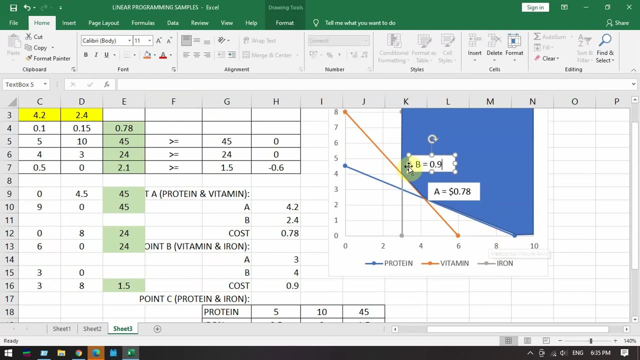 So meaning this is this point. Okay, so let's identify that as our point B. Okay, so B is equals to. we have computed it: it's equals to 0.9.. Okay, so we're talking about the cost here. that's why it's in dollar sign. 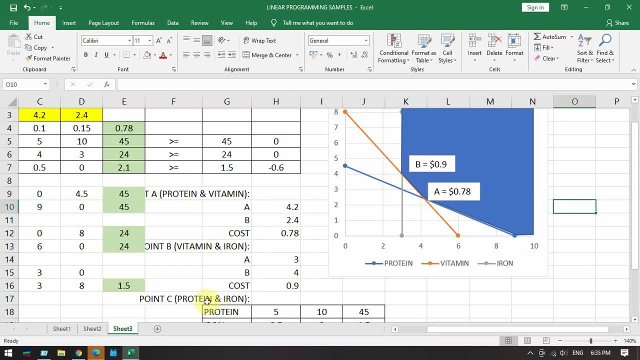 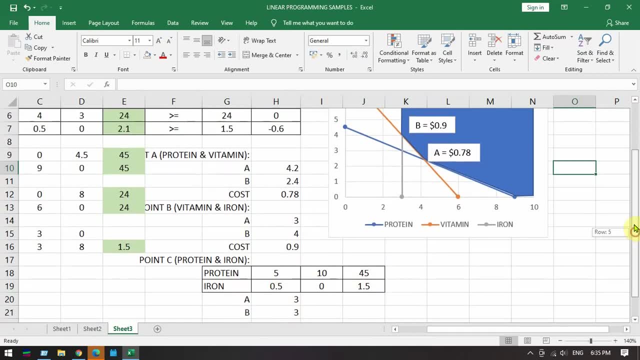 So this is this one. this is point A, Okay, And then our point C is where protein and iron intercepts. So that is where A and B are both in 3.. Okay, so that is this 3.. So this one. 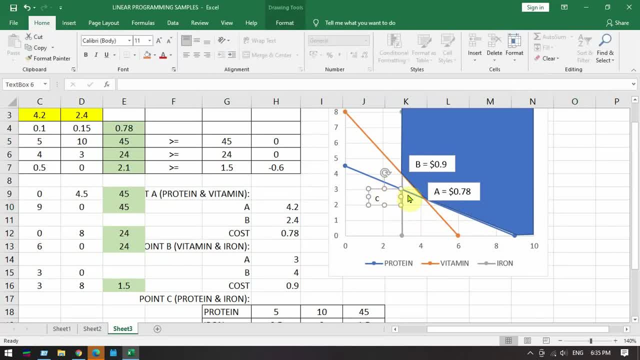 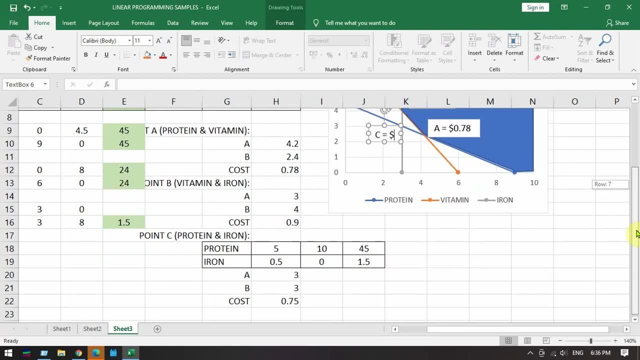 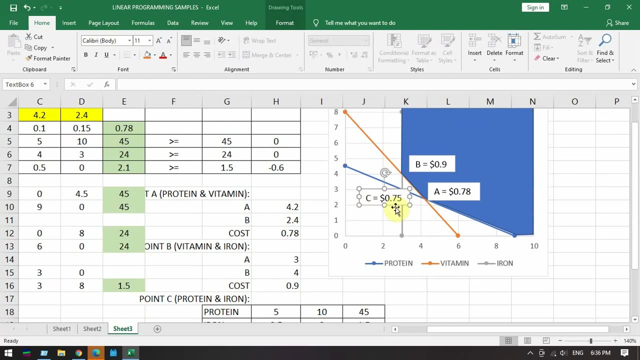 So this is our point C, And that is equals to 0.75.. All right, okay, so that's it. so that is our point C. So we have three options now for our optimal solution. So which is now our optimal solution? 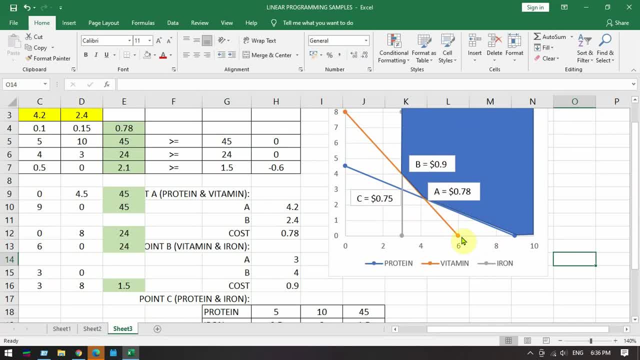 So, looking at this graph, okay, what we need is the point that is the lowest but should still be in the feasible region that we have identified. Point C is already outside our feasible region, So this is not our optimal solution. Point B is higher than A. 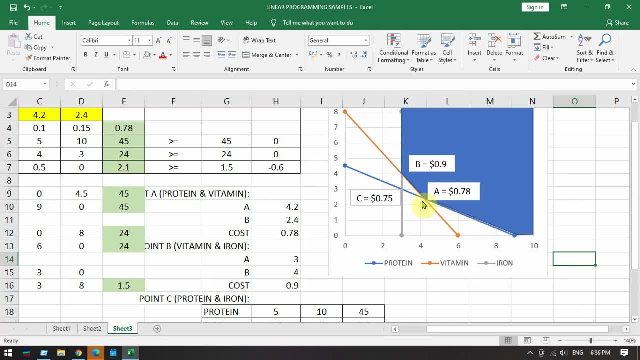 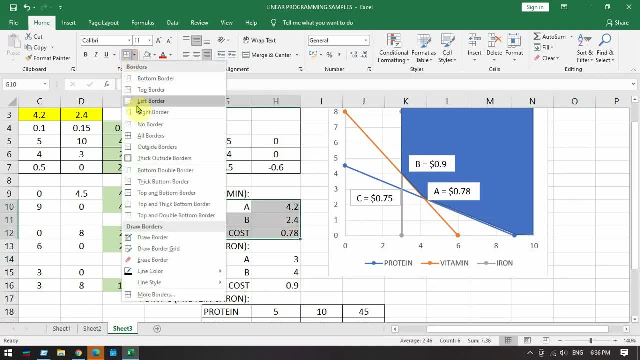 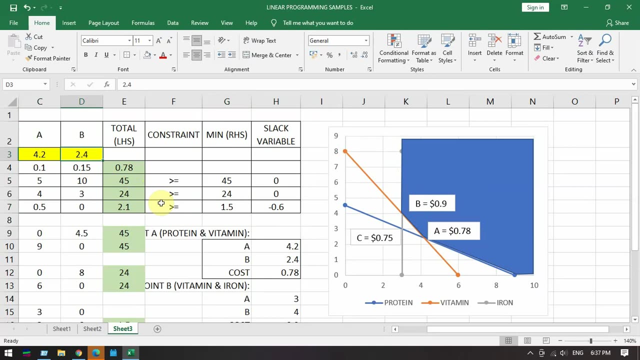 So therefore, A, which is still in our feasible region, is our optimal solution. So this should match, okay, our answer with the solver. Okay, where A is 4.2 and B is 2.4, and then we get. 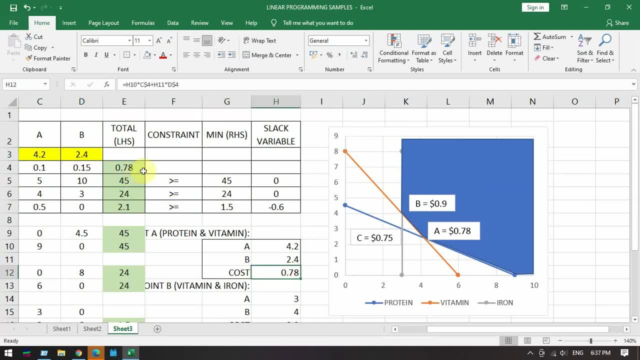 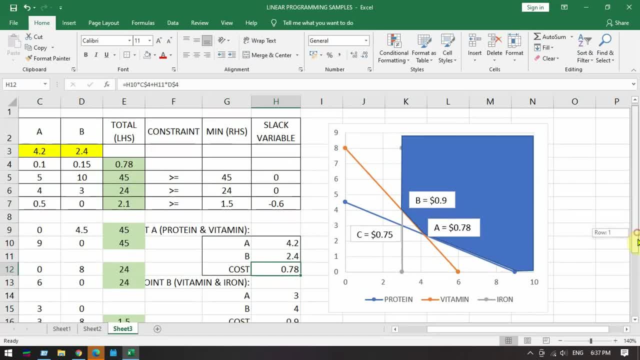 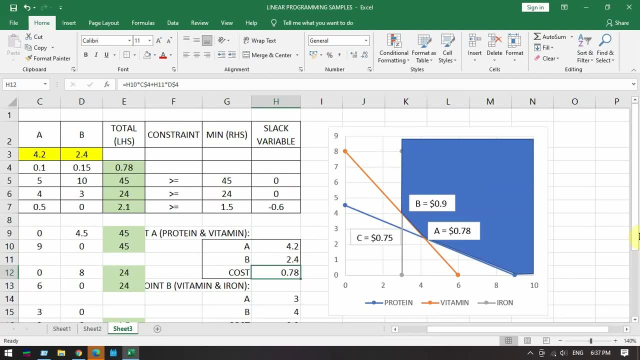 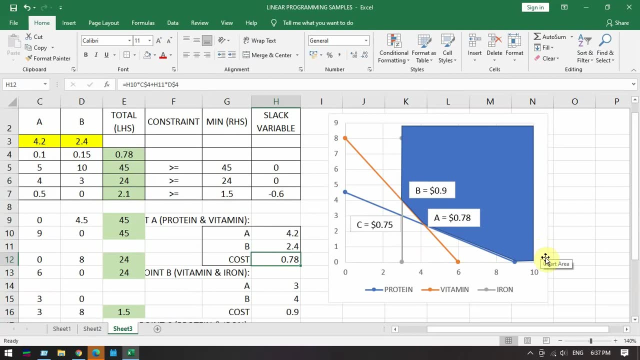 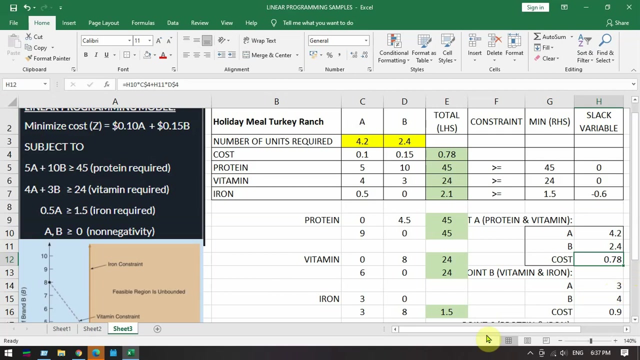 And this is it for minimization problem. Okay again, even if we use solver, we still need to solve our graph in this way. So and this is it. Let me know if you have any questions or concerns regarding this problem. okay.